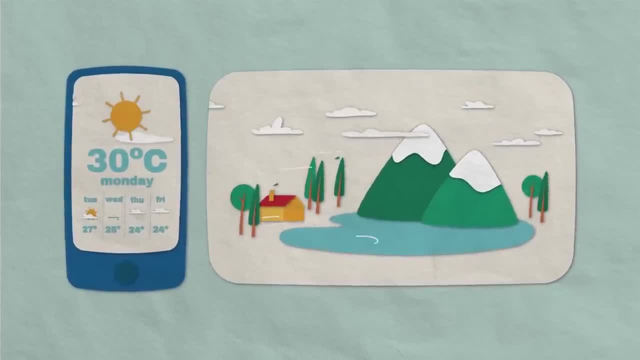 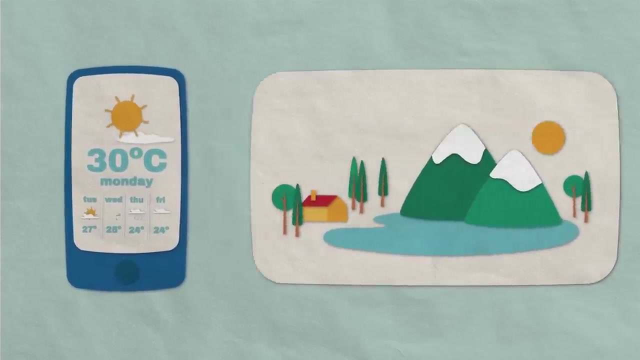 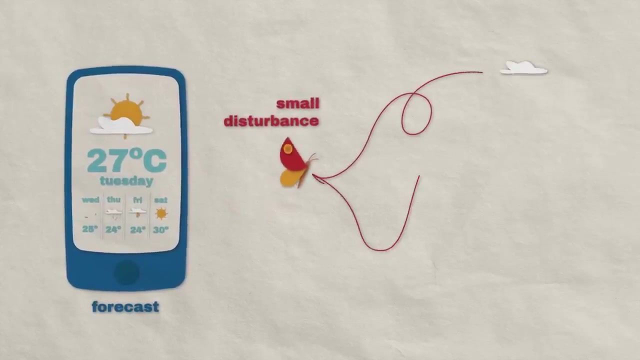 Unfortunately, there's something stopping this global web of data from producing a perfect prediction. Weather is a fundamentally chaotic system. This means it's incredibly sensitive and impossible to perfectly forecast without absolute knowledge of all the system's elements. In a period of just 10 days, even incredibly small disturbances can massively impact atmospheric. 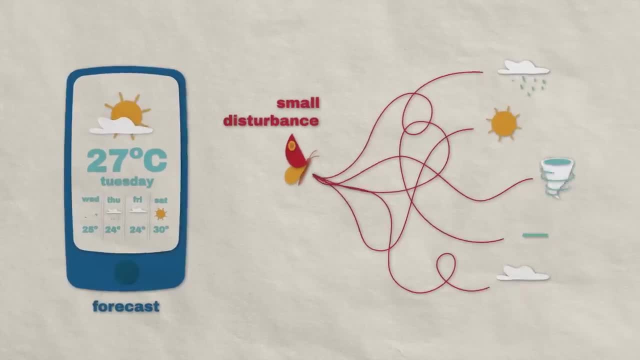 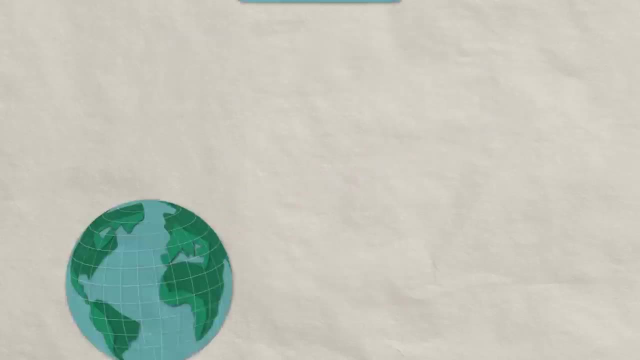 conditions In a period of just 10 days. even incredibly small disturbances can massively impact atmospheric conditions. Climate prediction, on the other hand, is far less turbulent. This is partly because a region's climate is, by definition, the average of all its weather data, But also 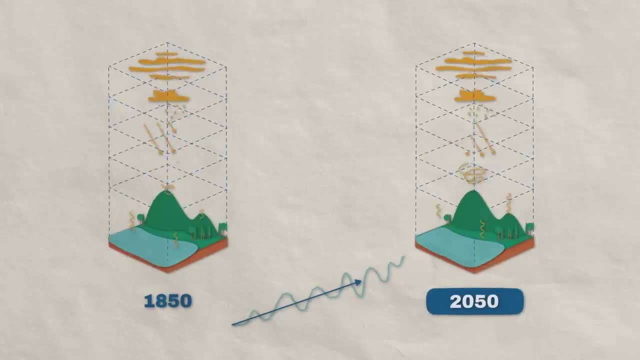 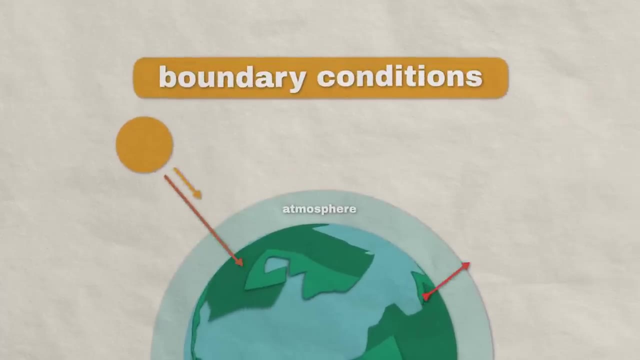 because climate forecasts ignore what's currently happening in the atmosphere and focus on the range of what could happen. These parameters are known as boundary conditions and, as their name suggests, they act as constraints on climate and weather. One example of a boundary condition is solar radiation. 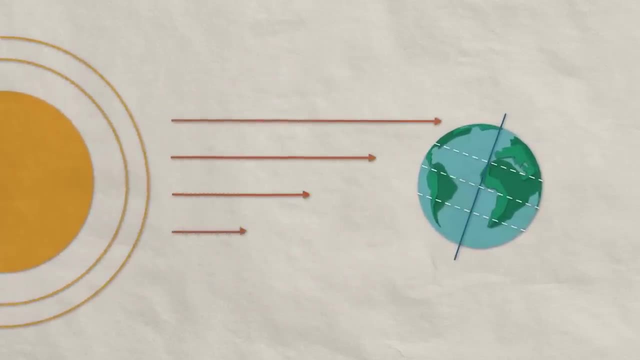 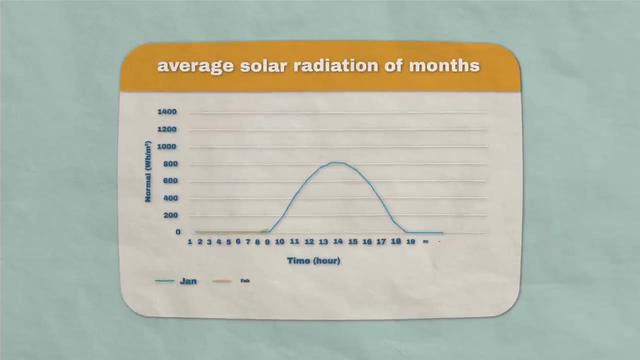 By analyzing the precise distance and angle between a location and the sun, we can determine the amount of heat that area will receive And since we know how the sun behaves throughout the year, we can accurately predict its effects on temperature, Averaged across years of data. 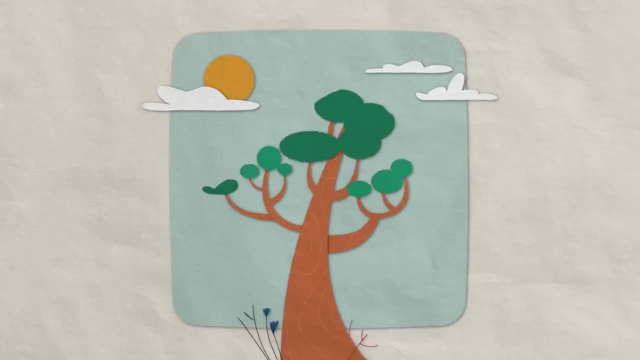 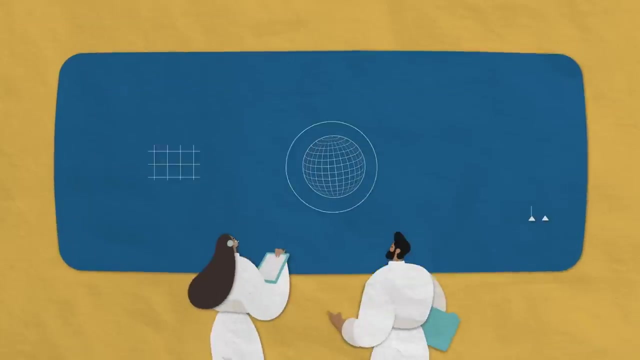 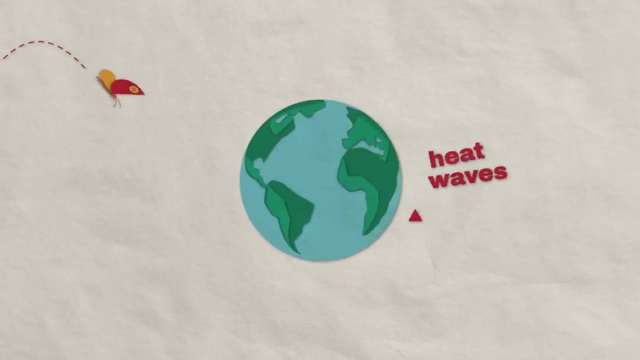 this reveals periodic patterns, including seasons. Most boundary conditions have well-defined values that change slowly, if at all. This allows researchers to reliably predict climate years into the future. But here's where it gets tricky. Even the slightest change in these boundary conditions 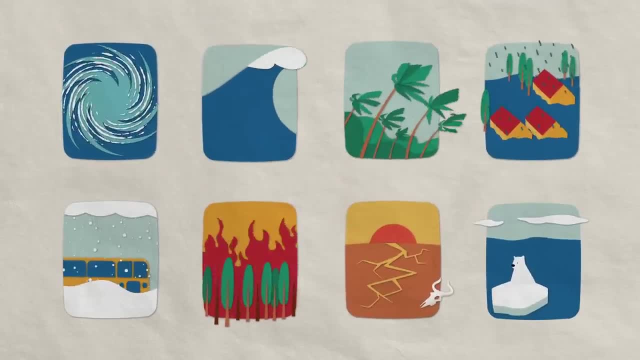 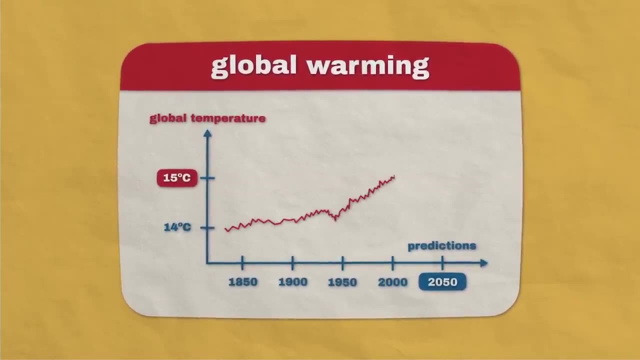 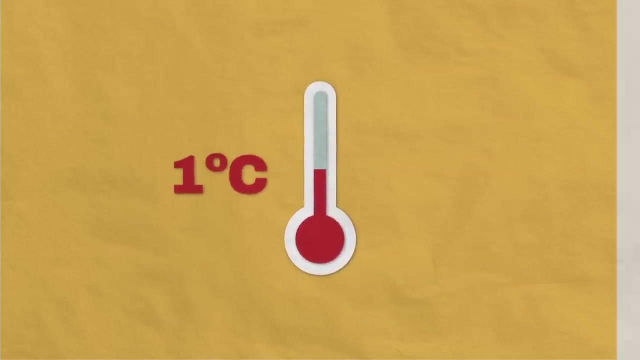 represents a much larger shift for the chaotic weather system. For example, Earth's surface temperature has warmed by almost 1 degree Celsius over the last 150 years. This might seem like a minor shift, but this one-degree change has added the energy equivalent. 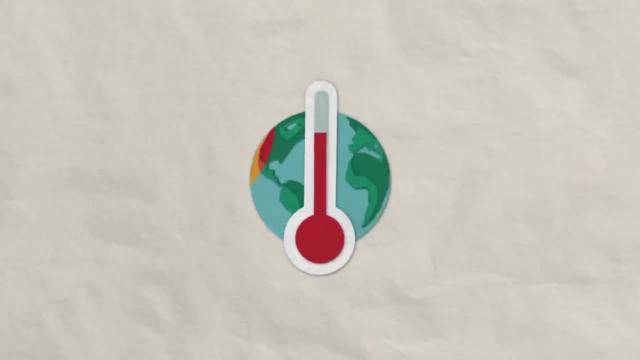 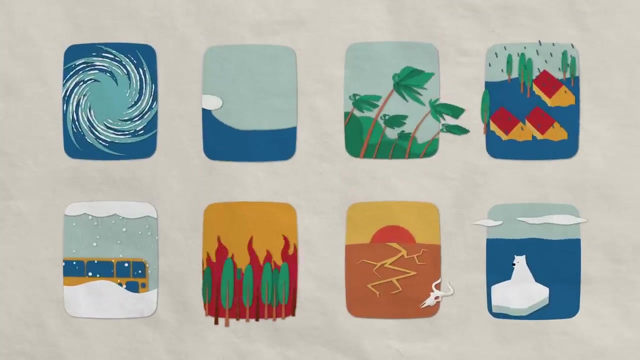 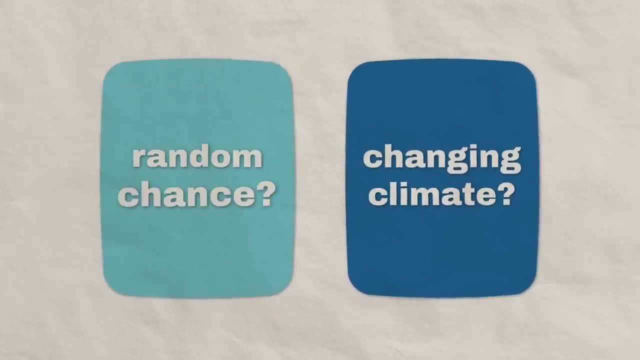 of roughly one million nuclear warheads into the atmosphere. This massive surge of energy has already led to a dramatic increase in the number of heat waves, droughts and storm surges. So is the increase in extreme weather due to random chance or changing climate.